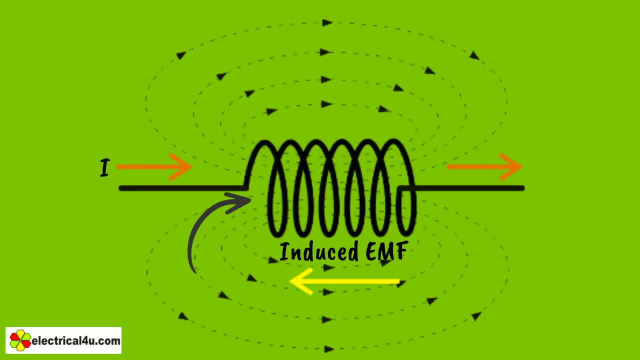 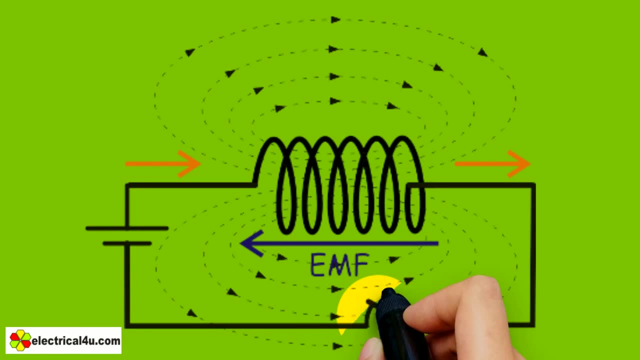 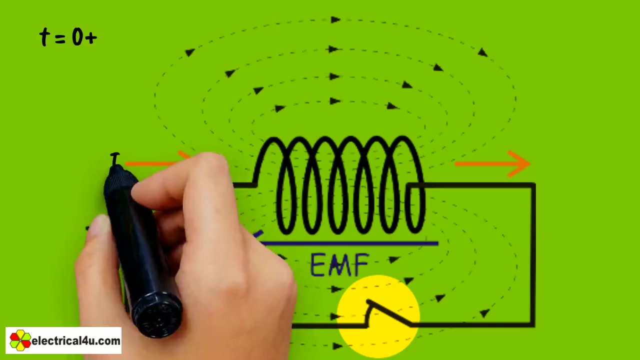 of change of current in that coil For the DC source when the switch is on, ie just at T, is equal to zero plus a current will flow from its zero value to a certain value And with respect to time there will be a rate of change in current momentarily. 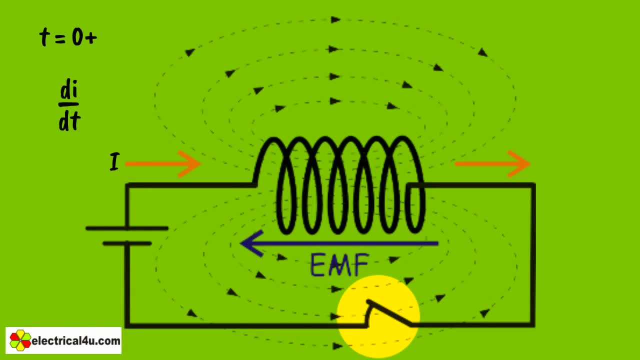 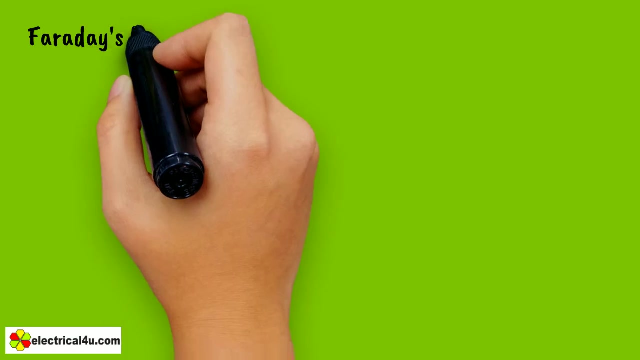 This current produces magnetic field lines, phi, through this coil As current changes its value to zero to a certain value. that's why magnetic flux phi gets rate of change with respect to the time That is d, phi, dt. Now apply Faraday's law in this coil. 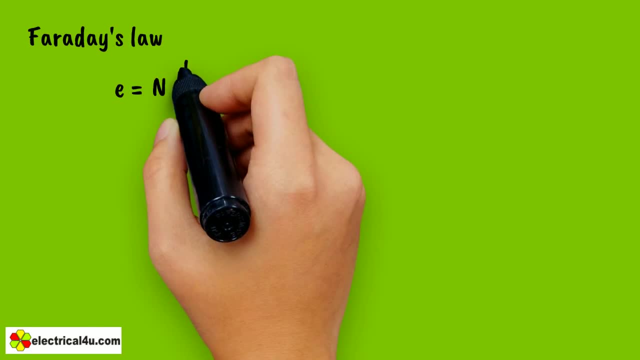 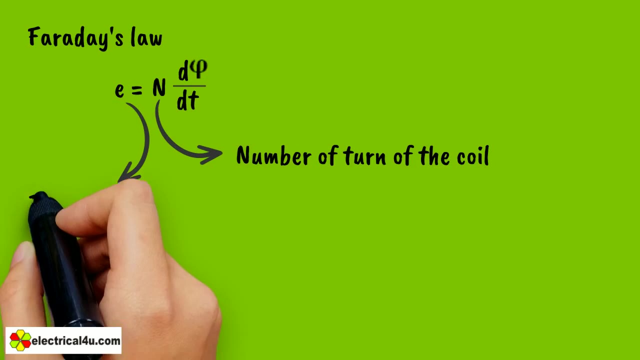 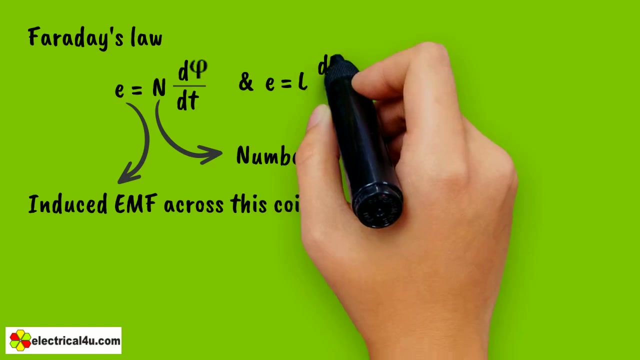 E equals n, d phi, dt, where n is the number of turns of the coil and E is the induced EMF across this coil: L di dt. E equals n d phi, dt. L i is equal to n phi, which is again equal to n into b, into a, where b is the flux density. 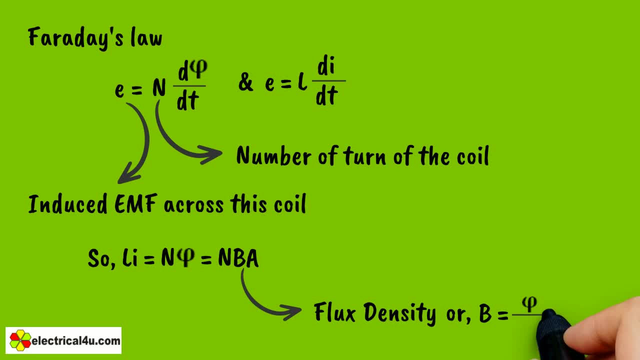 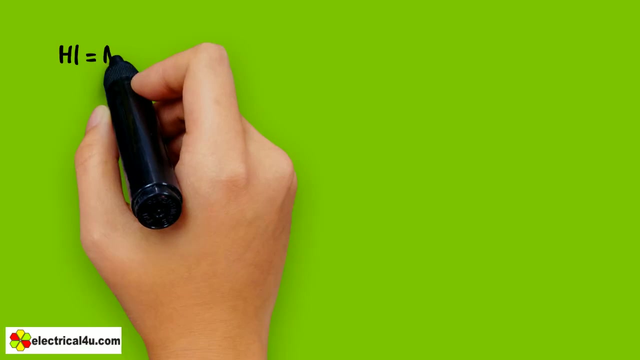 that is, b equals phi a divided by d, where a is the area of the coil. This n? phi or L? i, is called magnetic flux linkage and is denoted by psi. Again, H? L is equal to n? i, where H is the magnetizing force due to which the current will flow. This n phi is equal to n? i, where h is the magnetic flux density. that is, b equal to n? i. Again, H? L is equal to n? i, where h is the magnetizing force due to which the current will flow across this coil.